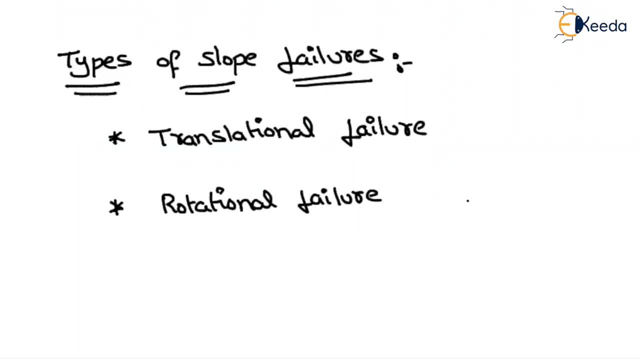 that soil mass will simply rotate with respect to some common point That is called the point of rotation. First, let us understand what is meant by a translation failure: Translation failure, Translation failure. Normally, this failure will observed in the infinitesimal. 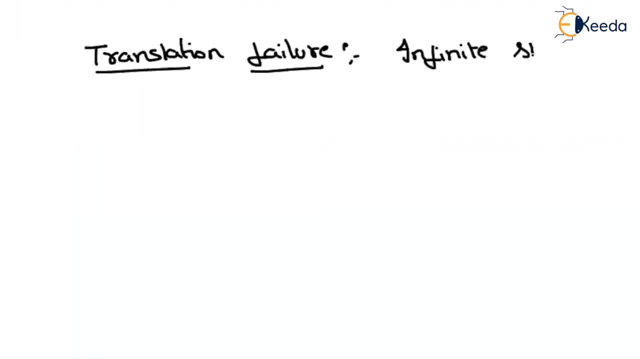 Yeah. So if this type of failure is considered as a surface, Yeah, In finite slope or a infinite flows. So if there is any infinite slope, then this type of failure we can see there. So let us leave the infinite slope. 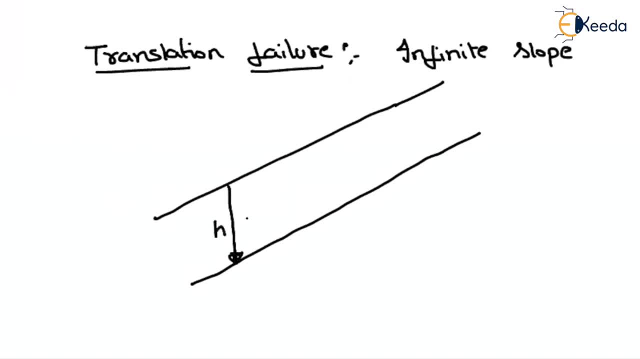 let us consider a slope that is extend a very long distance. okay, Then let us assume that. Consider a layer at distance of H. Let us say, on this layer, the shear stress acting on this layer, let us say this will be equal to tau And the strength of the soil along this layer will be S As. 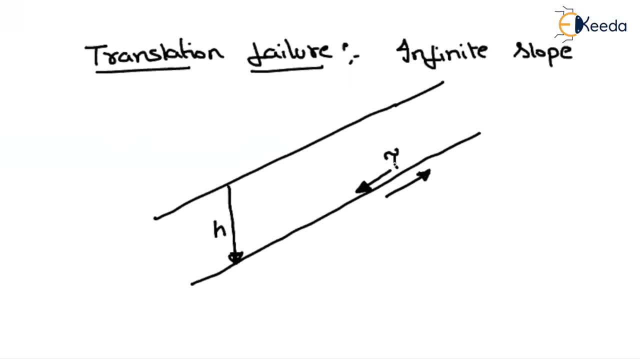 S is. tau is nothing but applied shear stress. this will try to cause this soil mass to move in the downward direction But as the soil having some shear capacity, this will try to restrain it. Let us assume that the shear strength of the soil along this layer will. 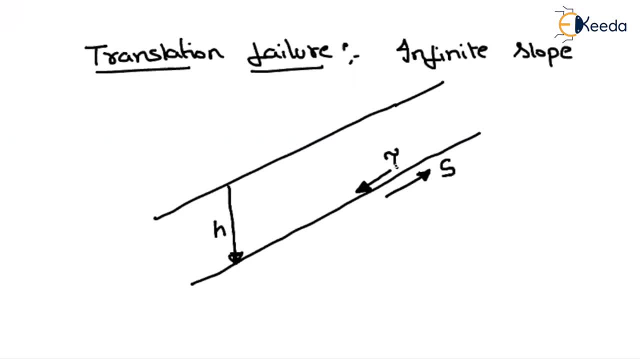 be S. So let us say: this is the applied force and this is the resisting force. So when this slope will be stable, as long as your shear strength is greater than the applied shear stress, then our slope will be stable. Once this shear strength is greater than the applied shear stress, then our slope will. 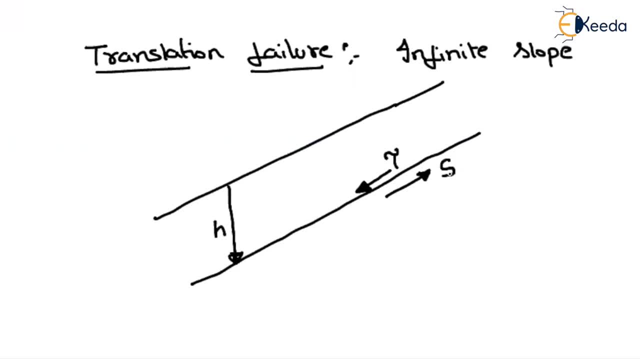 be stable. Once this shear strength is greater than the applied shear stress, then our slope will be stable. Once this shear strength is greater than the applied shear stress, if it exceeds the shear strength of the soil, then only translation failure occurs. That. 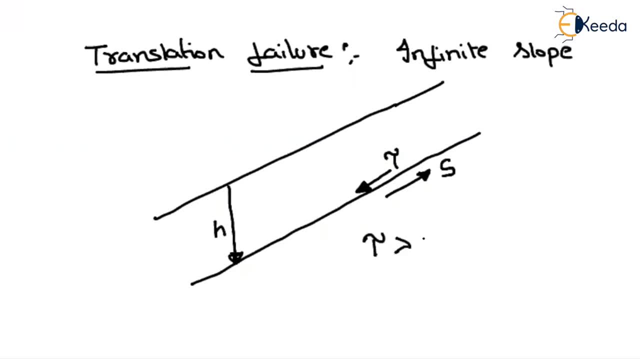 means if your tau, if it is greater than the S, then we can get the translational failure. Suppose, if you don't want any translational failure, that means to avoid failure of the soil, To avoid failure, whatever the shear stress that means, whatever the shear stress that. 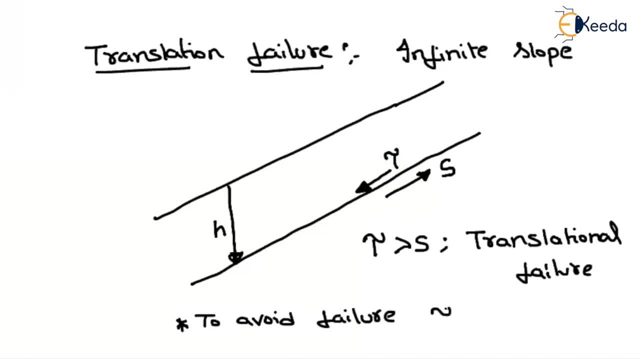 is acting on the depth H. let us say that I am calling it as a tau max to avoid the failure. the maximum shear stress acting on the infinite slope. that should be less than the shear strength capacity of the soil. So let us find out. factor of safety. Factor of safety is nothing but a. it is nothing. 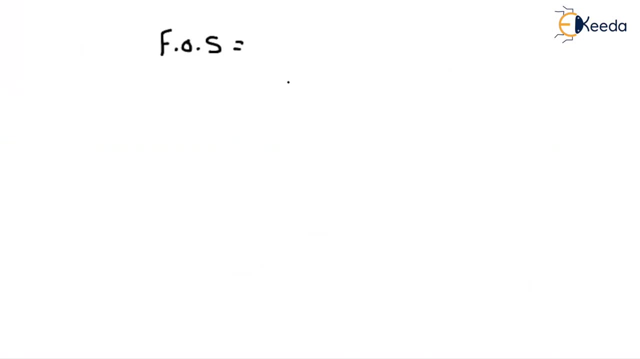 but a shear stress. Okay, So what is the shear strength of the soil denoted by S and whatever the shear stress acting on the layer that will be denoted as a tau, Suppose, if this factor of safety, if it is greater than one, that means your shear stress is less than the shear strength. 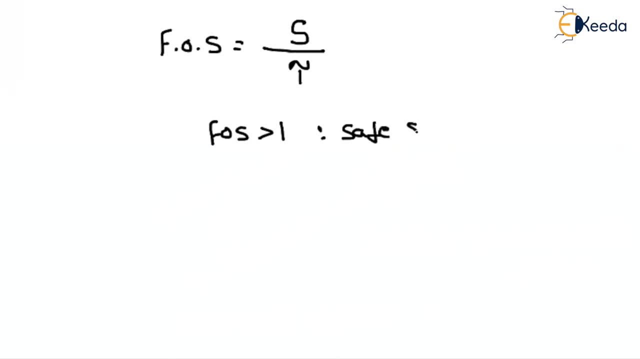 then we will call it as a safe slope. If your factor of safety, if it is coming less than one, that means Okay. If your applied shear stress it is coming greater than the shear strength capacity, then in this case the slope will be unsafe. 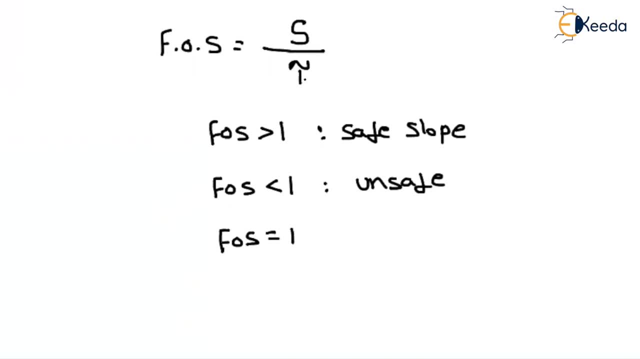 Suppose, if this factor of safety is equal to one, that means the applied shear stress is also equal to the shear strength capacity, Then we can say that it is under critical condition And also we can say that it is on the verge of failure. 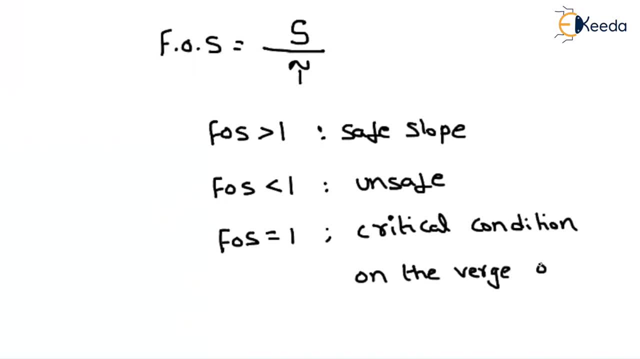 Okay, That means even if, after this factor of safety, that means if your shear stress is greater than just even by one mega Pascal or 0.1 mega Pascal, the slope will be failure. So that's what it is called. it is on the verge of failure, Even though, if small magnitude is increased, 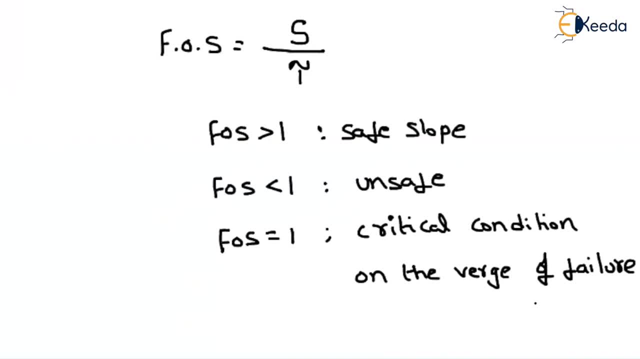 in the shear stress, the failure will occur. Now this is about the translational field. Okay, So for this stability of slope, we have to make sure that your shear strength capacity should be greater than the shear stress acting on the layer. 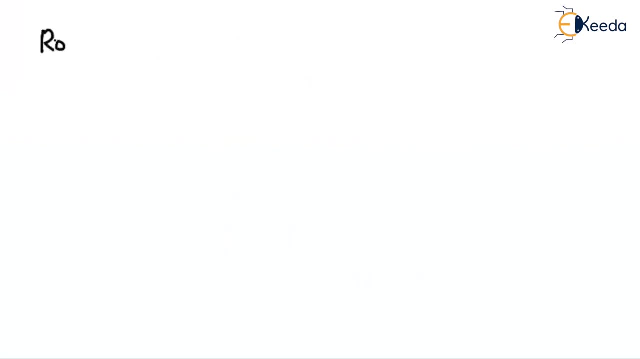 Now let us talk about the rotational failure, As we have already discussed rotational failure. normally this failure will observe in the finite slopes and also we will call it as a manmade slopes. The name itself implies that means whatever the soil mass that is going to failure. that 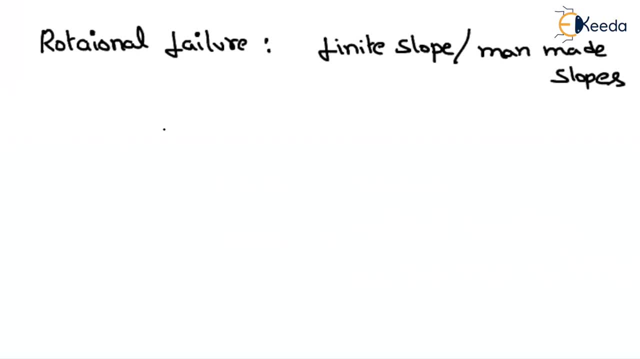 mass is simply going to rotate with respect to some common point that is called the point of rotation. So for that, let us consider an example, consider an embankment like this. Let us assume that this slope is of limited depth, Having magnitude h. then here suppose, let us assume that if this is the soil mass, that 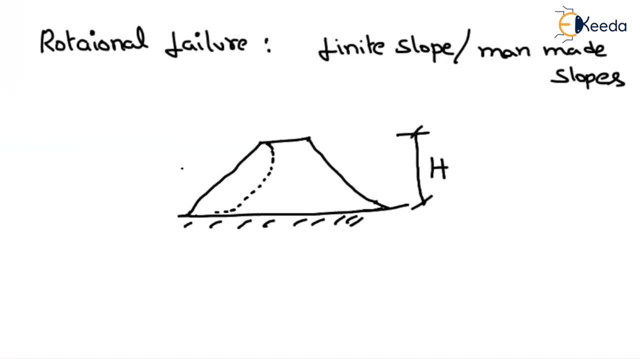 is going to be failure, then this whole soil mass will rotate with respect to some common point. So this point is called the point of rotation. So this whole mass, whatever I am hatching the area, this whole mass will simply rotate. 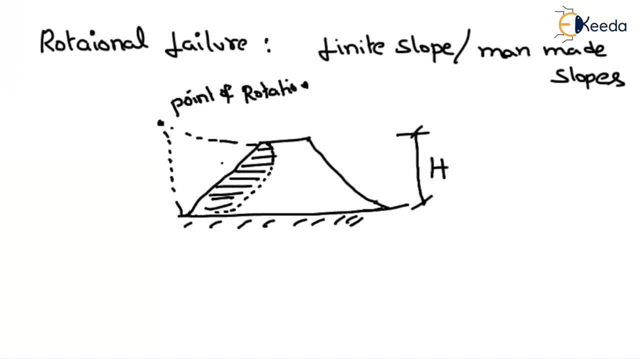 with respect to some common point, So that is why it is called the rotational failure, As the soil mass is rotating with respect to some common point, then here the factor of safety will be find out, based on the movement condition. So here we have to talk about the two different types of movement. 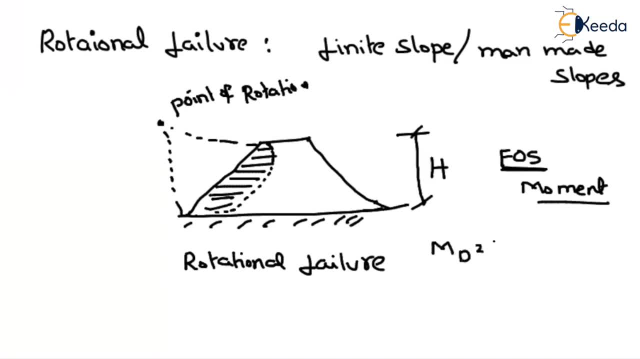 One is because of the- let us call as it is- MD. MD is nothing but a driving force. That means because of some external forces, or else we can call it as a disturbing forces. those forces will try to rotate the soil mass with respect to some point. 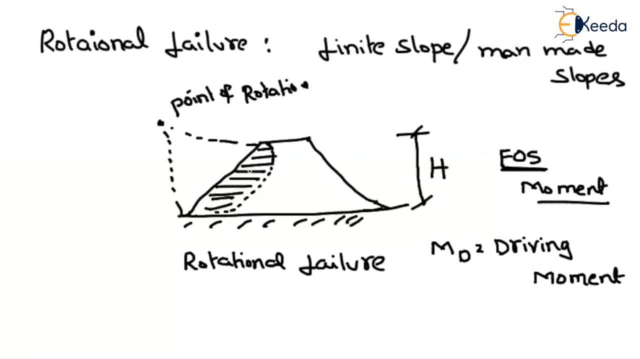 That means this movement is trying to cause the rotation of the soil mass. That is why it is called driving movement. As some applied forces are trying to rotate the soil mass at a same time as our soil is having some capacity, that soil mass will not be able to rotate. 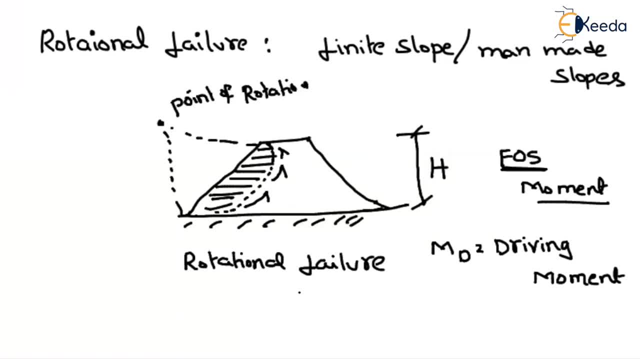 So that is why it is called driving movement. That is why our soil mass will try to restrict the movement. So what is that movement is called? that is called the rotation movement, or else we can call it as a resisting movement. This is developed from the sweet, as long as your driving movement is less than the resisting. 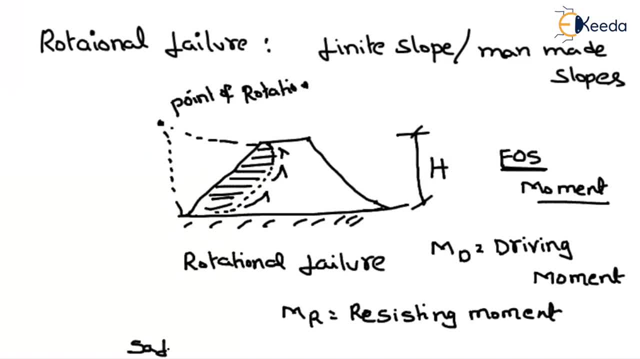 moment you were: slop Hayırl wierde. So either slope with脸 As long as you are driving, movement is less than the resisting movement, değil? você, fuck, Alex is does not want than the resisting moment. then we can call it as that. this slope will be failure slope. so from this. 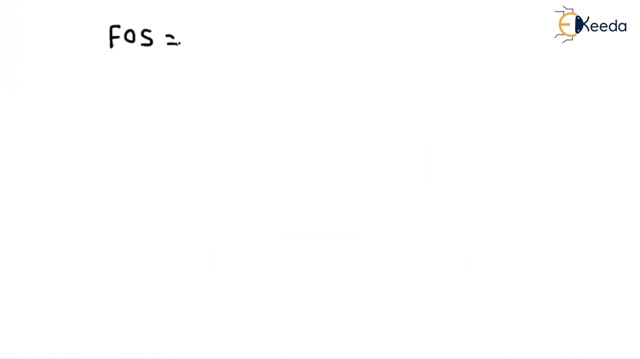 what can we call it as a factor of safety? factor of safety, it is nothing but called as a resisting moment divided by driving movement. so, just like in the previous case, if your factor of safety, if it is coming, greater than one, then we can say that the slope will be unsafe. that means 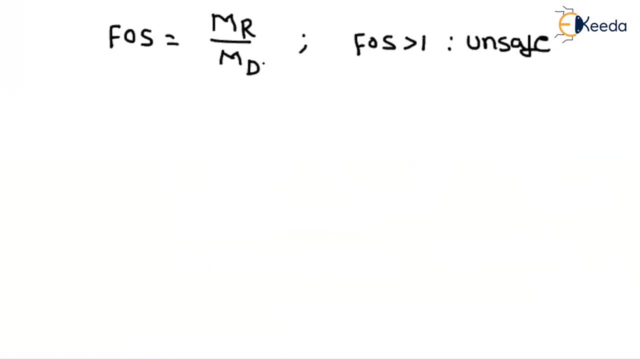 the resisting movement should be greater than the driving movement and also in this, under this, rotational failure there may be. if we go in sub classification, there may be three different types of failure can occur. so again, i will classify this rotational failure into three different categories. that means one is nothing but a tau failure and another one is nothing but a. 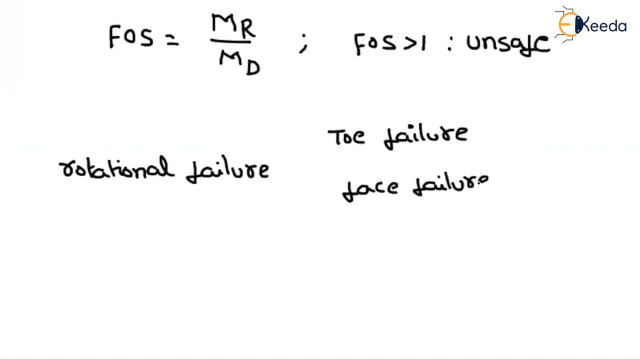 phase failure and another one is nothing but a base failure. again, from the name itself we can understand that means: if it is a tau failure, the failure mass will pass through the tau point. if it is a phase failure, the failure mass will cut along the face of the slope. if it is a base failure, the failure slope will cut along the base. 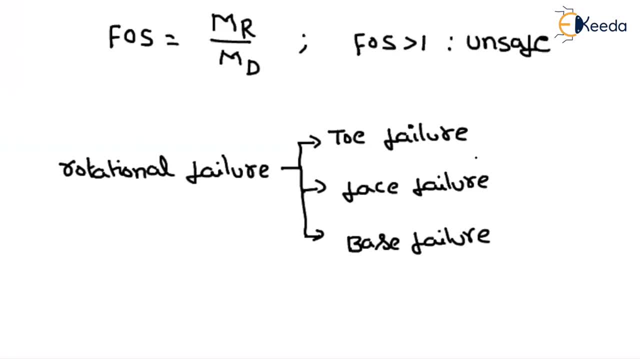 so this is the failure mass. this type of classification we can identify depending upon the depth factor. so from the magnitude of depth factor we can identify which type of failure is going to be happen. so for the understand, let us consider again an embankment and also let us consider there is a some hard surface. 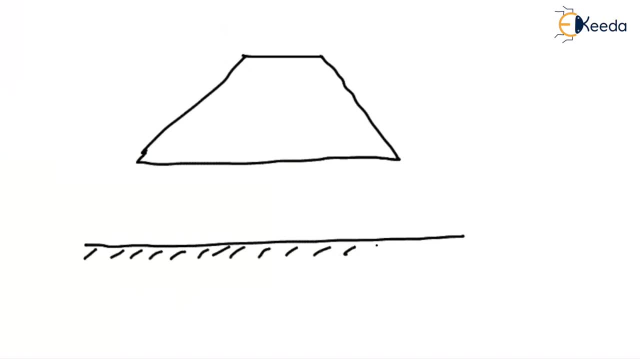 below the base of the embankment at some distance, x. let us say this distance is nothing but a, d and let us say this is nothing but a ground surface, ground level and the height of the embankment. let us consider the height of the embankment. 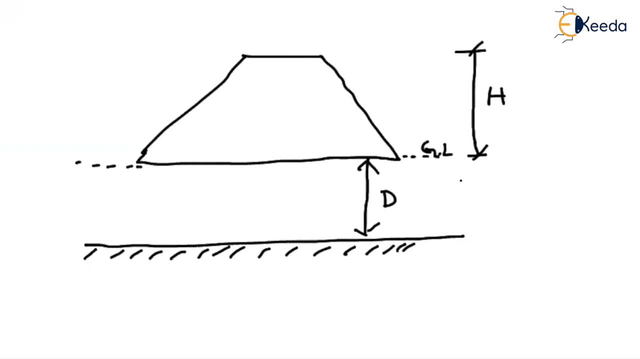 is nothing but a h. okay, the depth factor, that means the depth factor will be defined. i am writing it as a d, subscript f. that will be defined as a h plus d greater than the power of the force 3 divided by H. So if this depth factor, if it is greater than 1, then we may have. 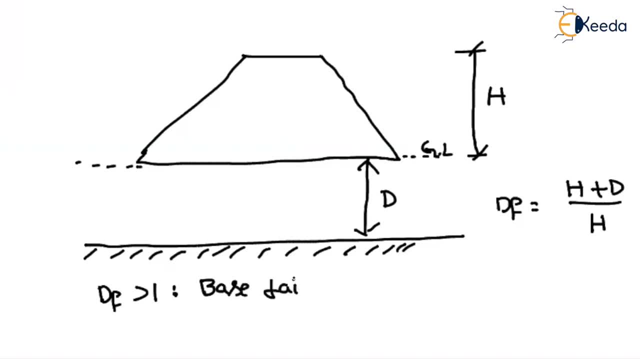 the base failure. That means how the rotation of mass will happen. The rotation of the mass that will going to happen like this. That means the rotation of the soil mass will touch the below the ground level surface. So this is called the base failure Normally. 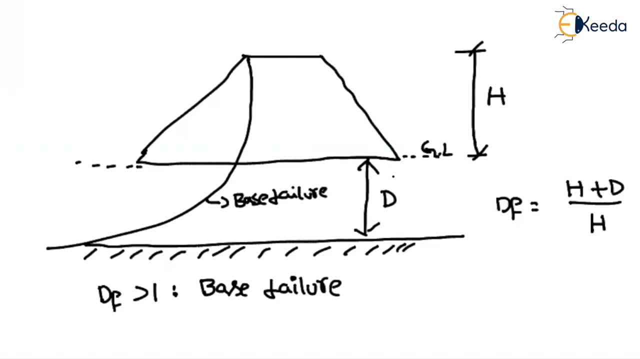 this type of failure will occur when, below the ground level, the soil is very, very small. In that case only we can have the base failure. So what about the second case? If your depth factor, if it is equal to 1, then we may observe the toe failure. That means 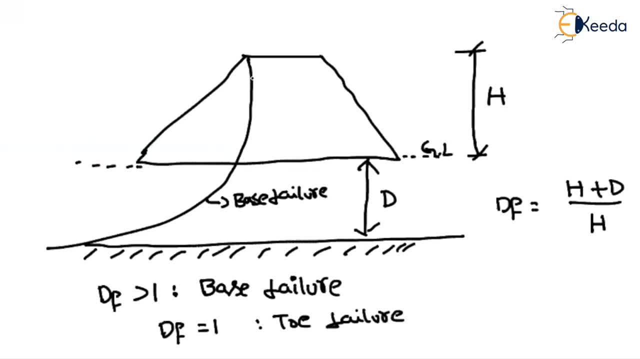 whatever the soil mass, that is failure. that point is passing through the toe of the embankment. What is the toe of the embankment? This point, So the failure's mass slope that pass through the toe point. So this one is called it as a toe failure. So, similarly, the another factor, 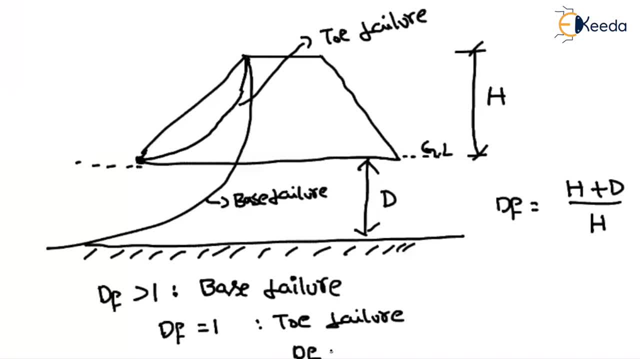 that means if your depth factor, if it is coming less than 1, then it is called as a face failure. That means whatever the soil mass that is going to fail, that is cutting or passing through the face of the embankment. So if the soil mass failure happen like this, then 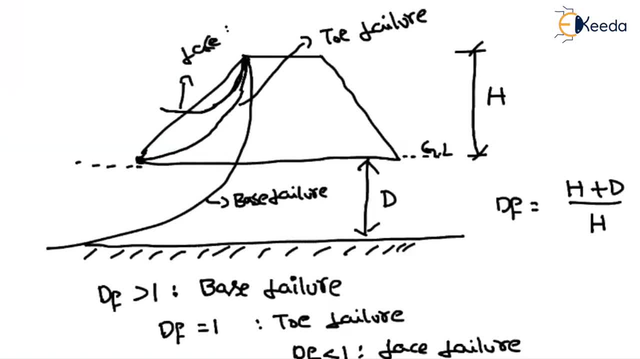 this will call it as a face failure. So, depending upon this depth factor, we can identify which type of failure is going to happen in the or under the rotational failure. Now, that is it about the types of slope failures. In the next class we will study about the stability. of the infinite slopes. Thank you,